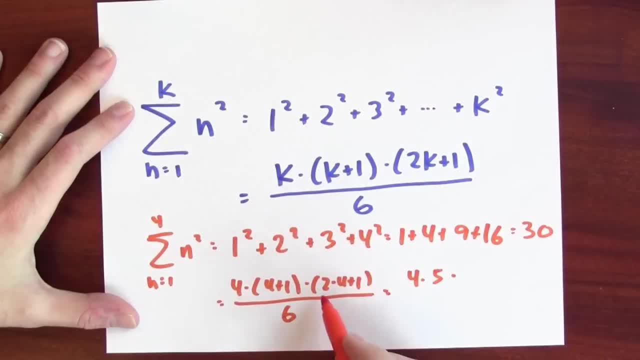 Well, that's 4 times 5 times 2 times 4 plus 1 is 9 divided by 6.. 6 is 2 times 3, so the 2 kills part of the 4 and part of the 9.. 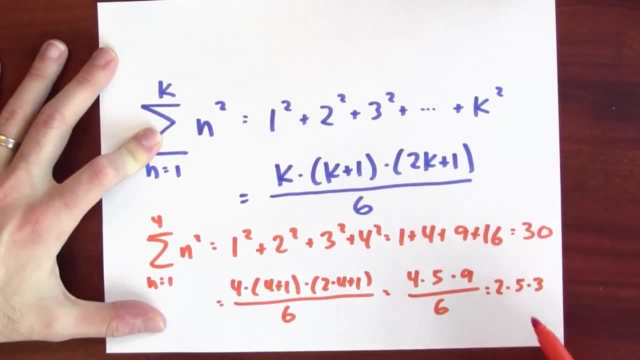 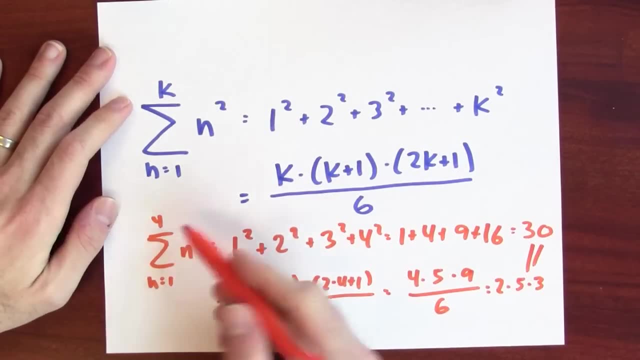 To give me 2 times 5 times 3.. And yeah, I mean 5 times 3 is 15.. Twice 15 is 30.. It really works, at least for the value 4.. Of course, this isn't a proof in general. 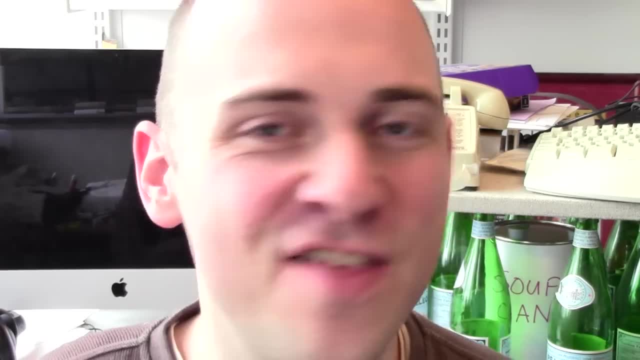 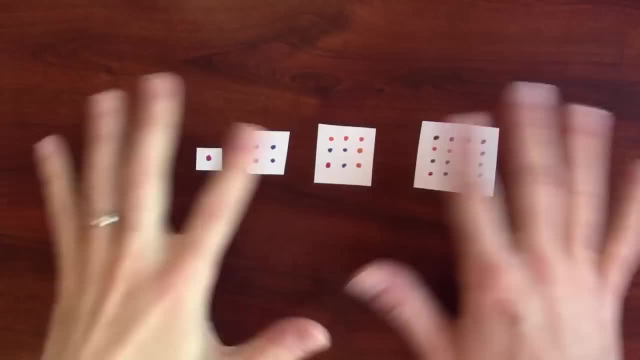 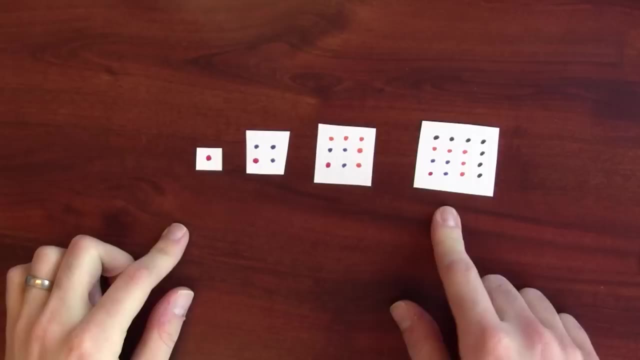 so how am I going to verify that that statement is true? Well, one argument is a geometric argument, really a proof by picture. So here's a geometric or a diagrammatic way of writing down 1 squared plus 2 squared plus 3 squared plus 4 squared. Now I know there's 30 dots here, right? 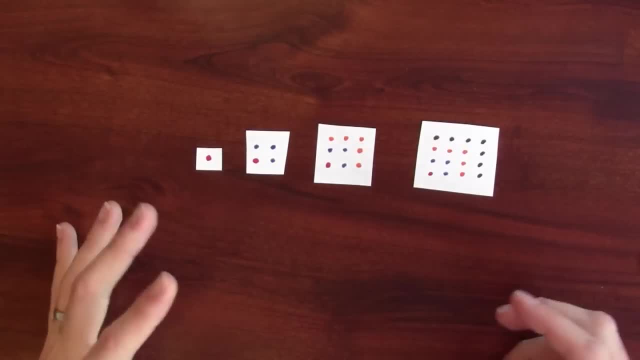 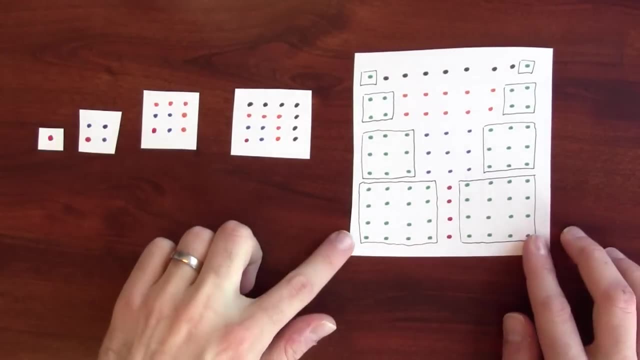 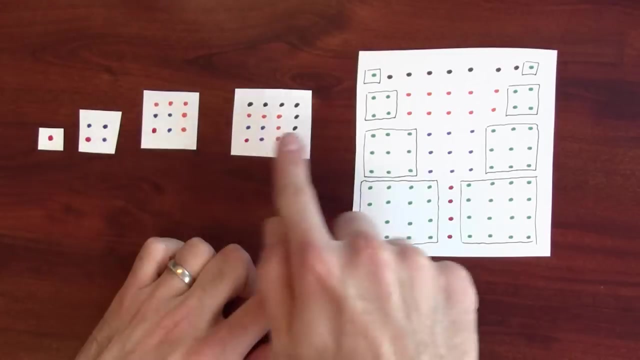 But I'm trying to draw a diagram that suggests the general pattern. Okay, so let's try to add up these, these four numbers. I'm going to use this device. I'm going to use this device here. What is this? Well, what I've done here is I've taken 3 copies of these k squares, right? 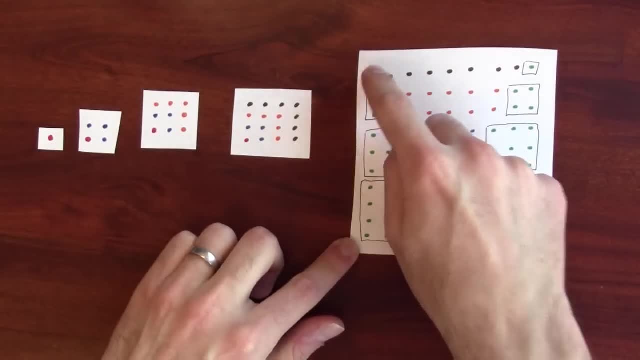 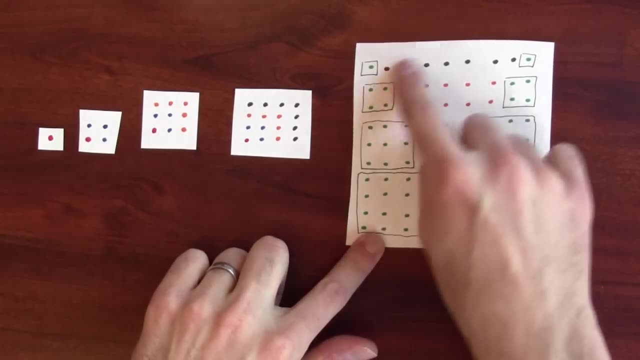 So here's 1 squared plus 2 squared plus 3 squared plus 4 squared. Here's another 1 squared plus 2 squared plus 3 squared plus 4 squared, And in the middle I sort of mixed it up a bit. 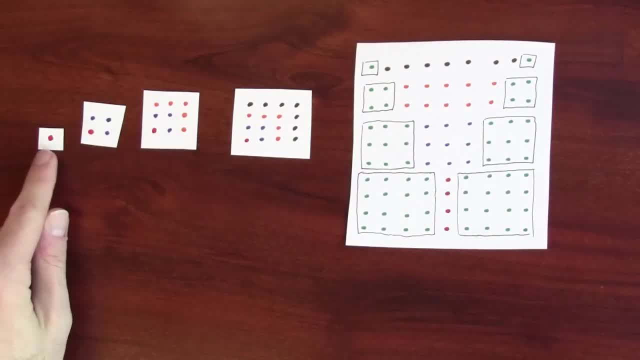 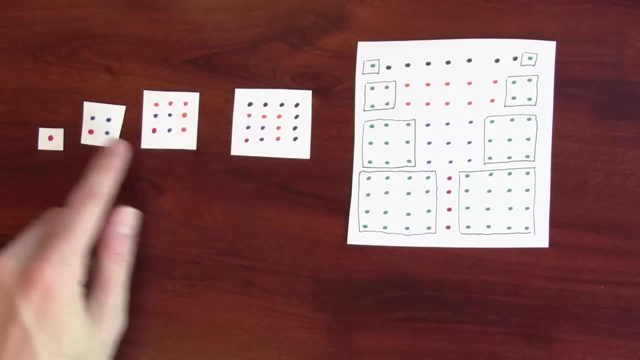 I've taken the lower left-hand corner dot which is red, and I've lined them up vertically here. I've taken the next sort of third and the next sort of three long L shape which I've drawn in blue here, and I've 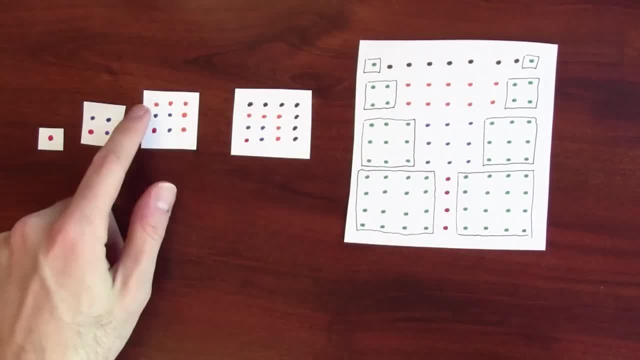 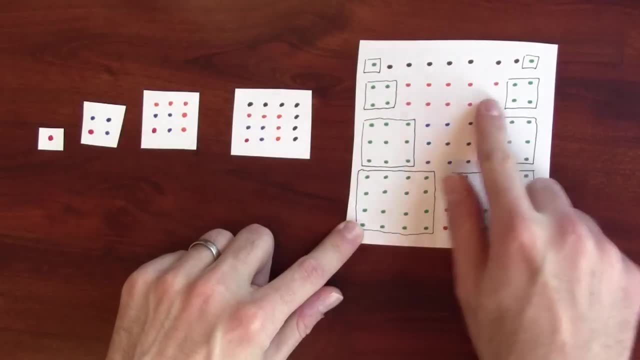 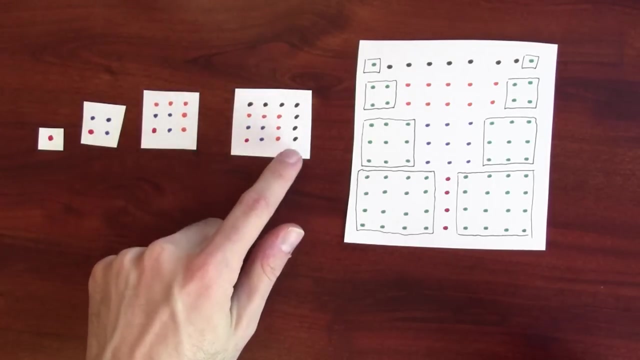 straightened them out and placed those three here. I've taken the two five long orange L's and straightened them out here And then here at the top I've got one long brown L comprised of seven dots and I've straightened that out right here at the top. 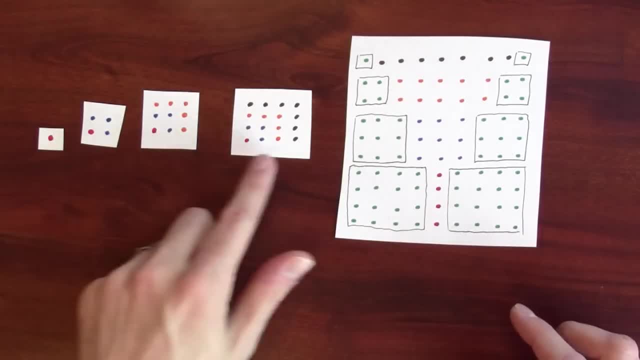 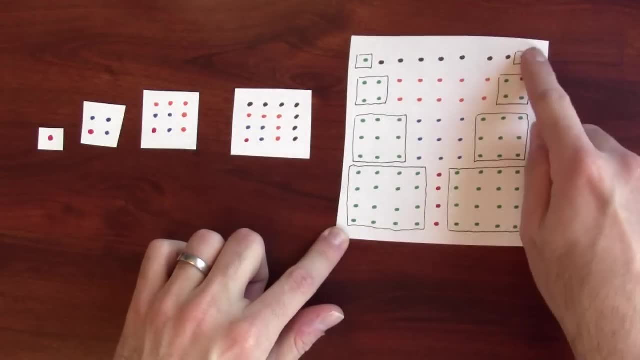 So what's happened here? right, I've taken three copies of my sums of squares, right? So I've got three copies of all these squares. One set is down here, one set's down here and the other set is mixed in the middle. 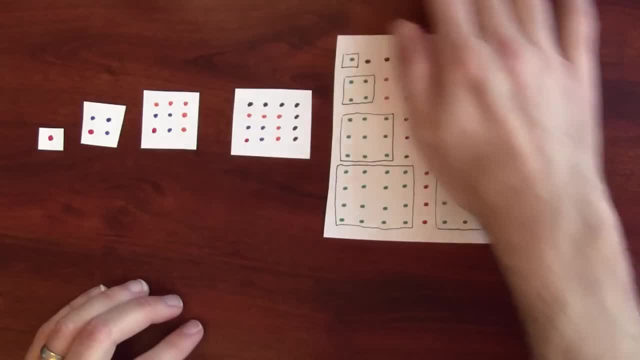 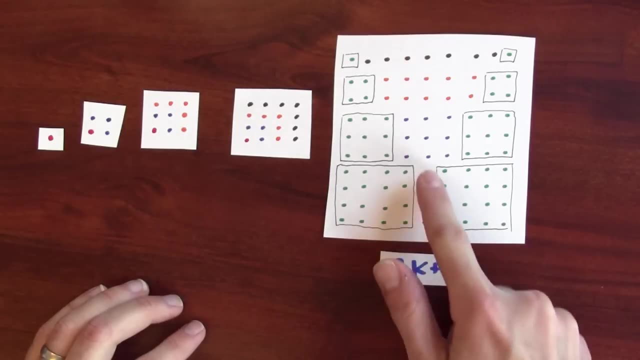 And now I can figure out how big of a rectangle this is. Well, the bottom here. this is a k by k square, k by k square, and these are built out of the corners. They're just one dot, So this whole bottom side is made up of a square. 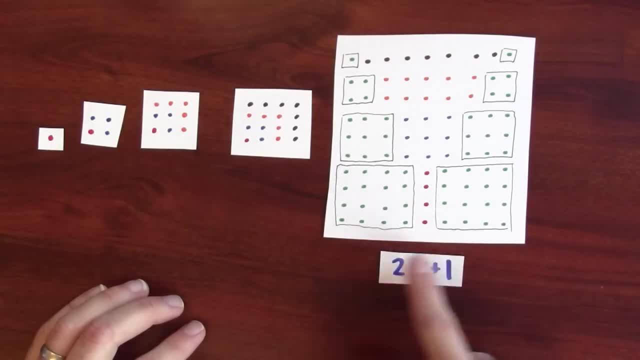 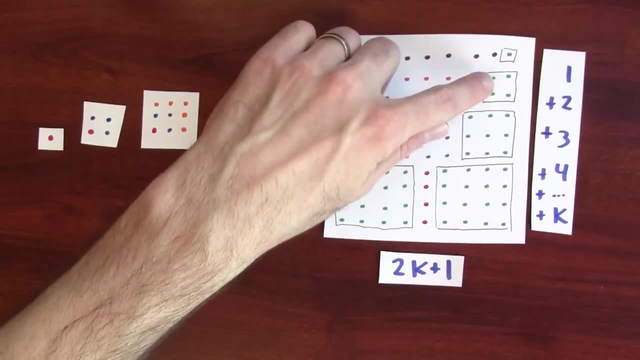 This whole side is made up of two k plus one dots, k plus one plus k, or two k plus one. What about along the other side? Well, along the other side I've got one dot plus two dots plus three dots plus. 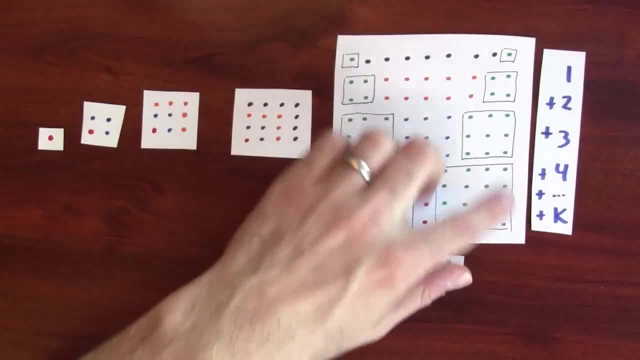 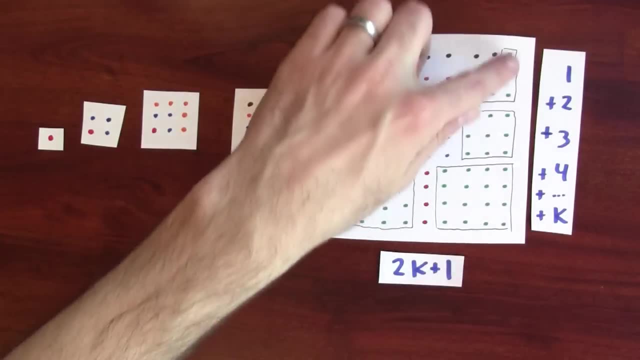 four dots, And of course this is just a a specific picture. So in general it'd be one plus two plus three plus four plus that, until I get to k Right. So I have to figure out how tall this rectangle is. but I in fact know a formula for one plus two plus three plus four up. 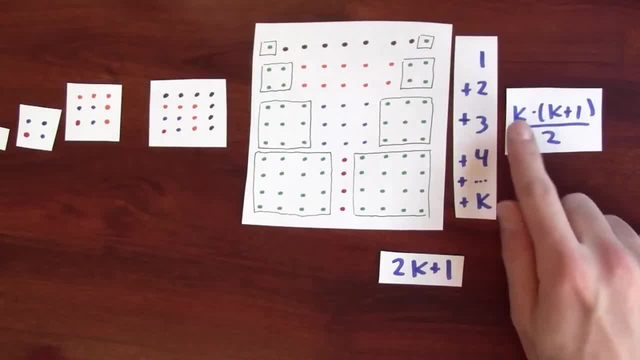 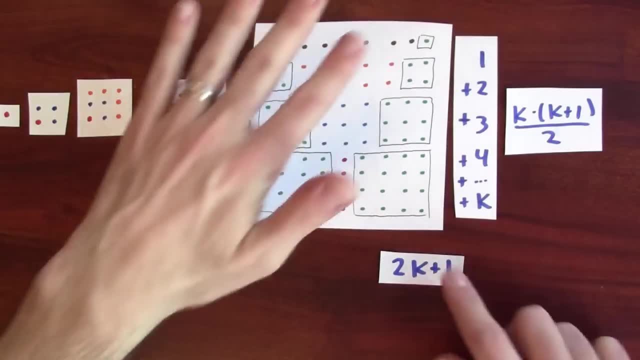 through k right, We figured that out already: It's k times k plus one over two. So I've taken three copies and built them into a rectangle whose base is two k plus one and which is k times k plus one over two tall. 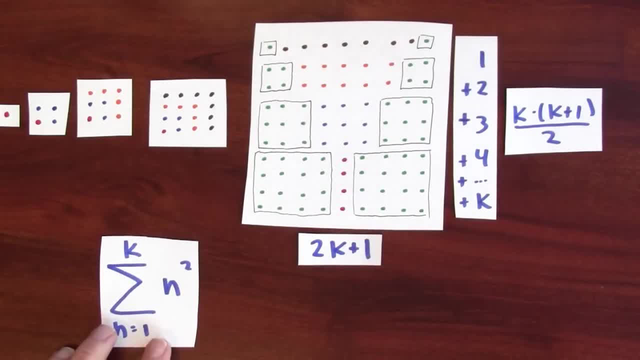 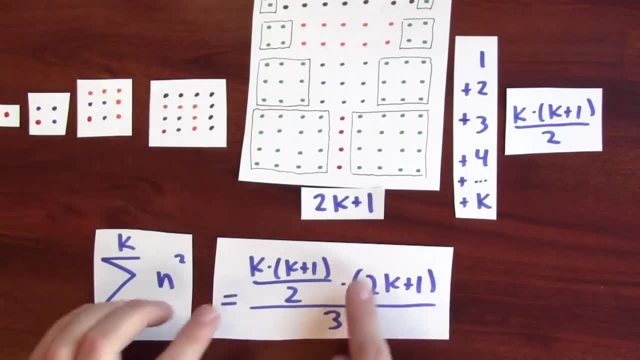 So that means that this sum, which is what I'm trying to compute, must be: well, it's the the height of this rectangle times the width of this rectangle divided by three, Since I used three copies of of these squares to build the big rectangle. 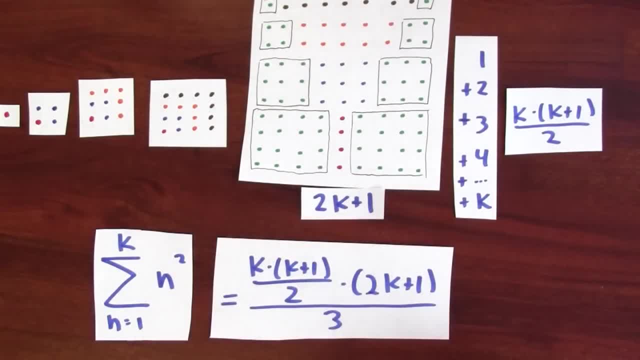 So I end up dividing by three, And this is in fact the formula that we had right. The original formula was k times k plus one times two, k plus one, all over six. But that's just a rearranged version of this formula. There are other geometric arguments, as: 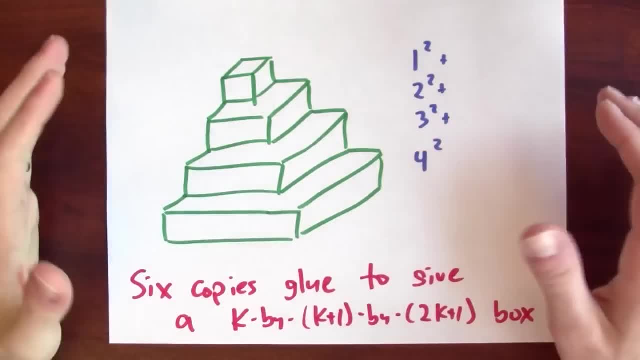 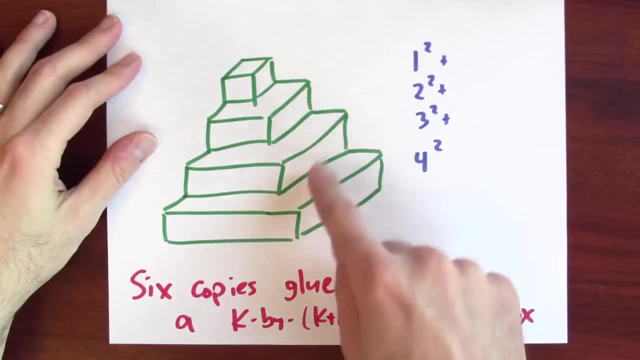 well other proofs by picture that you could give, And there are other geometric arguments too. Here's another way to get at this sum of squares formula. I could write down my formula. I could write down my sum of squares as something built out of little tiny. 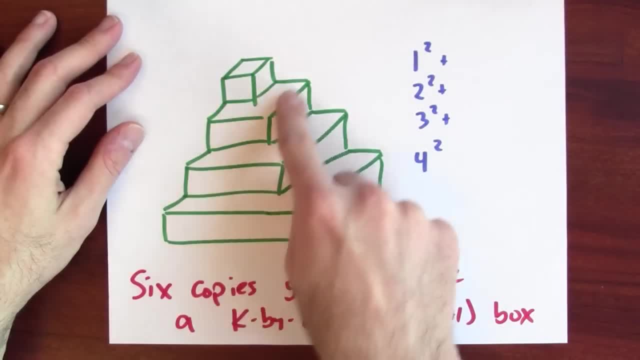 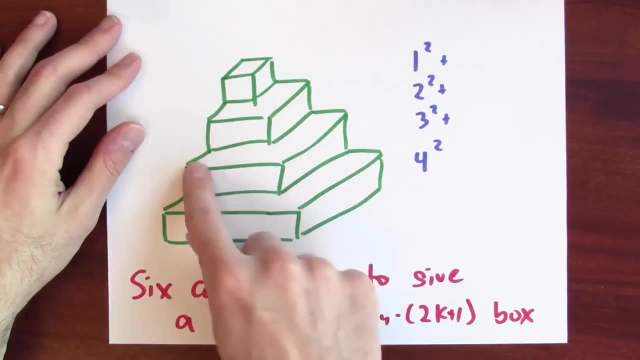 cubelets right Here. I've got one cube. Underneath I've got two squared cubes right, But this is a two by two by one block. Underneath I've got nine little cubes right. It's a three by three by one block.